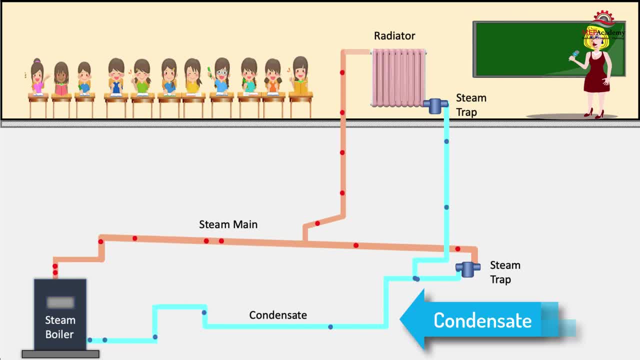 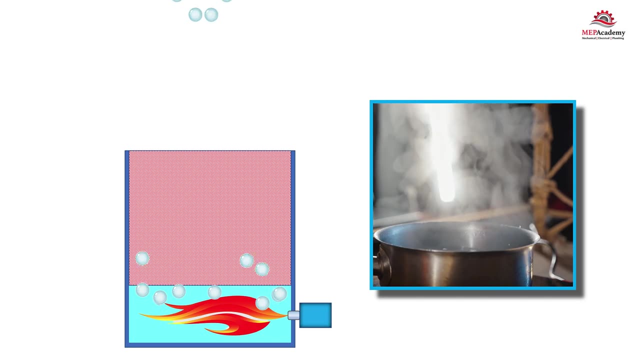 Condensate from the steam condensing needs to be brought back to the system for reuse. unless the steam is used for a process, The condensate can be brought back by gravity or with the use of a condensate return pump. When heat is added to water, its temperature will rise until it hits the point of evaporation. 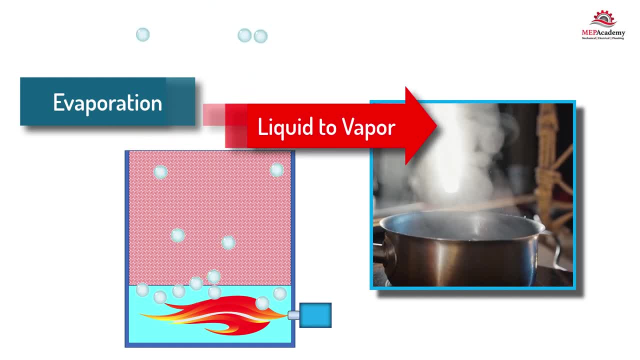 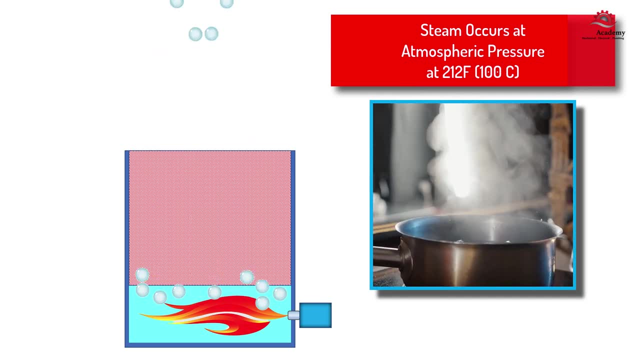 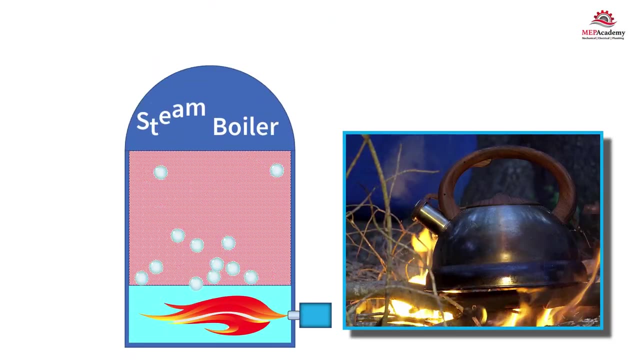 At this point it changes from a liquid into a vapor or steam. This occurs at 212 degrees Fahrenheit or 100 degrees Celsius At normal atmospheric pressure. If we enclose the water within a steam boiler with no opening to the atmosphere, the steam 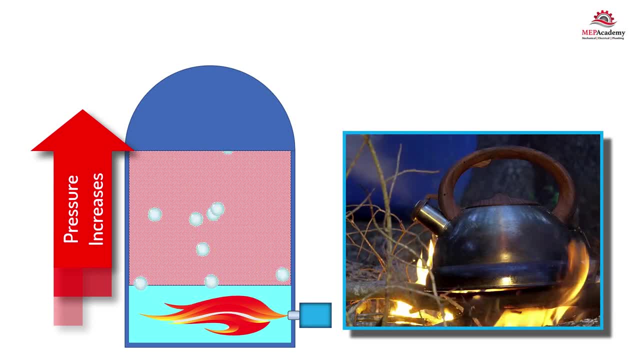 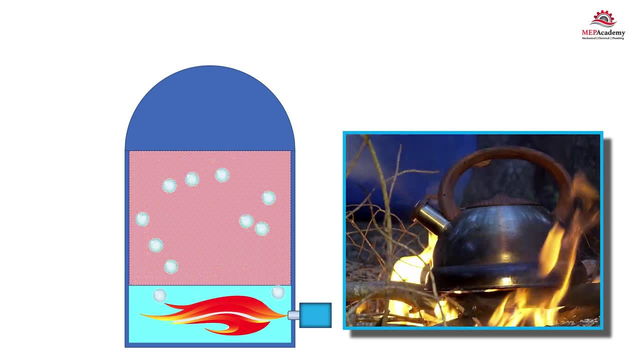 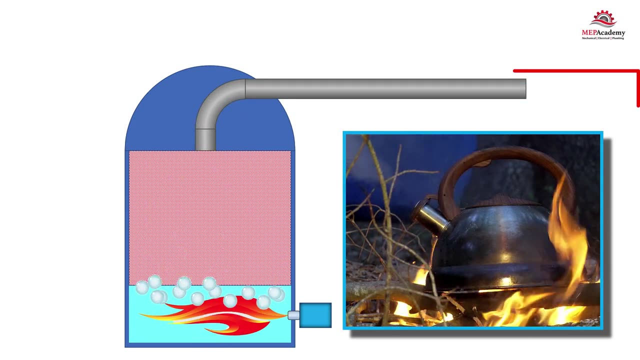 will increase the pressure within the system as the molecules move faster and faster, colliding into each other and the walls of the boiler, looking for a low pressure escape route, like the hole in the tea kettle If we connect piping to an opening in the steam boiler. 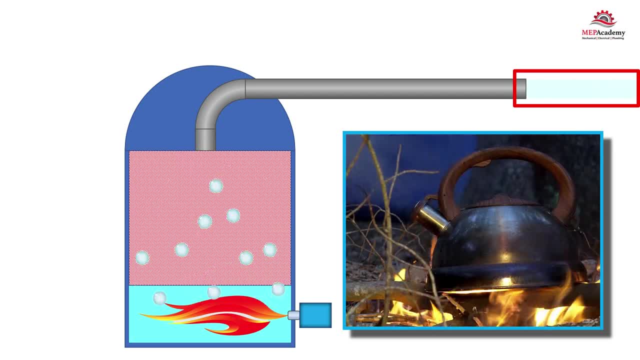 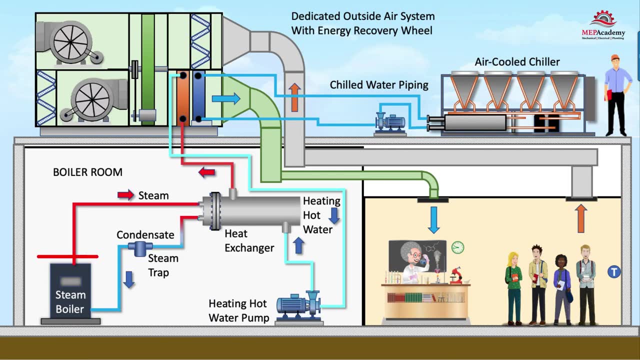 The steam will exit the boiler into the piping without the need of a pump, but just by the pressure created by the steam. Here we use a steam boiler to feed the primary side of a heat exchanger. The steam will transfer heat to the secondary loop, which is feeding the heating hot water. 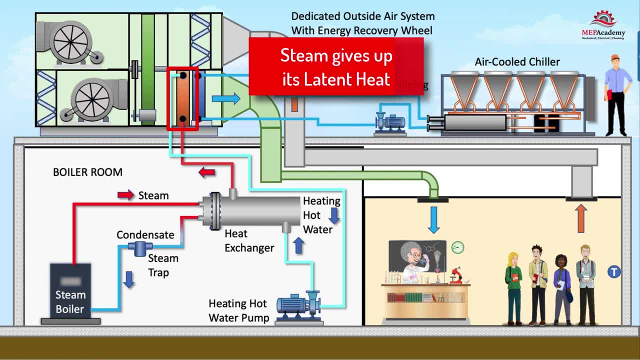 coils and air handlers. The steam gives up its latent heat and condenses as the heat is transferred to the secondary side of the heat exchanger. To make sure that we are not letting steam into the condensate- After the condensate return, we install a steam trap. 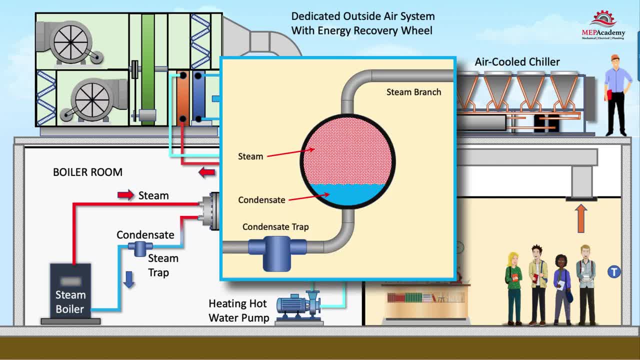 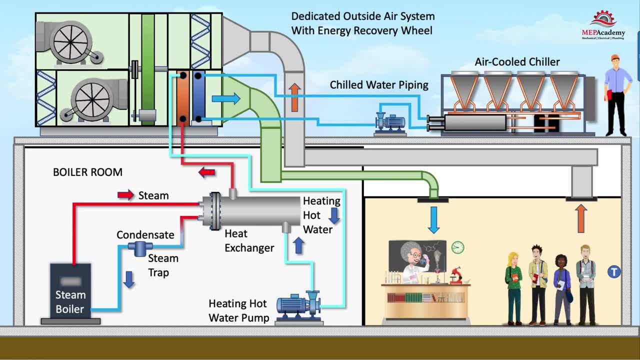 The steam trap prevents steam from passing through and only lets condensate through. On the secondary side of the heat exchanger is a separate loop of water that serves to heating the air in the building air handlers. If we look inside the heat exchanger we can see that the primary and secondary piping 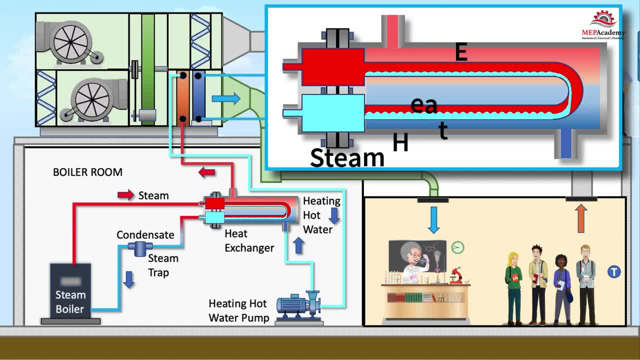 never mix. The steam enters the heat exchanger as steam and leaves as condensate While the secondary loop is not mixed. The secondary loop heating hot water is moved by a pump through the system. The secondary loop heating hot water returns, enters the bottom of the heat exchanger and 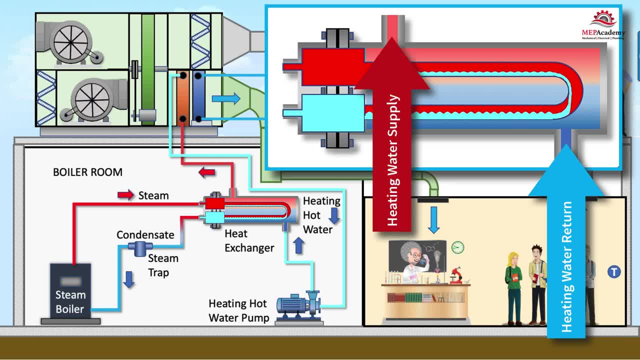 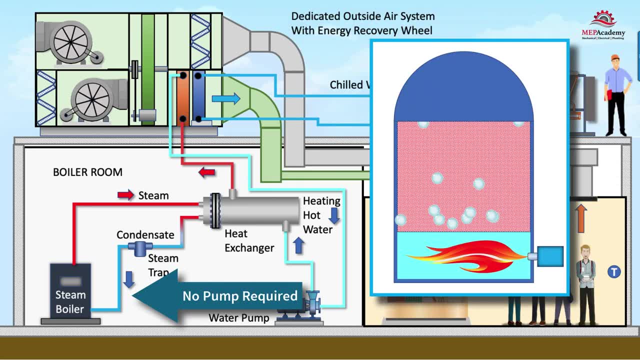 picks up heat from the steam and leaves through the top to the air handlers heating hot water coil. The steam boiler doesn't need a pump as the molecules are moving fast and exerts pressure on the walls of the boiler, and when the piping is connected to the boiler, then pressure 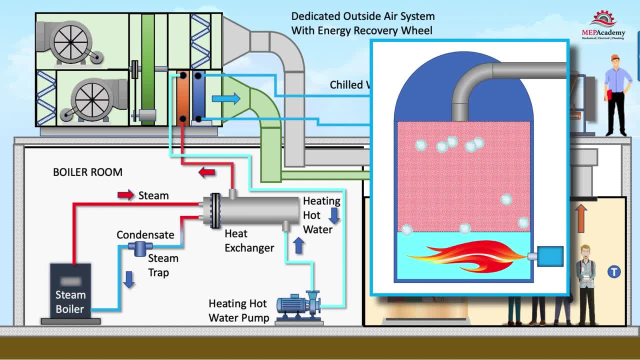 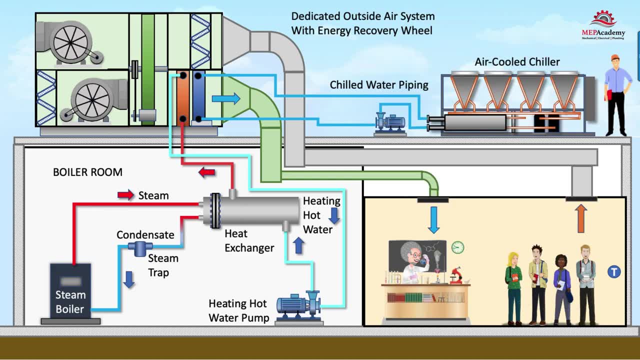 pushes the steam out of the boiler and into the pipes just like a teapot. Now the steam is escaping out of the spout, whistling as it exits. Now let's remove the professor and expand the equipment room to make room for a domestic. 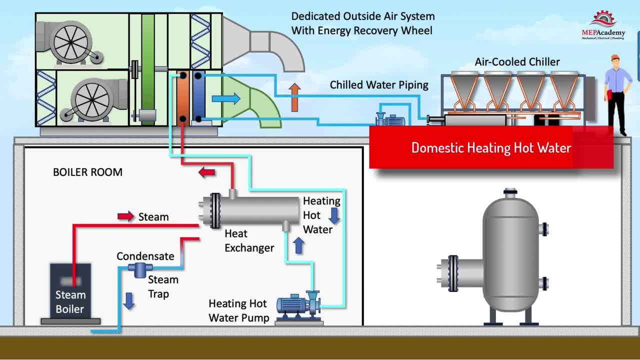 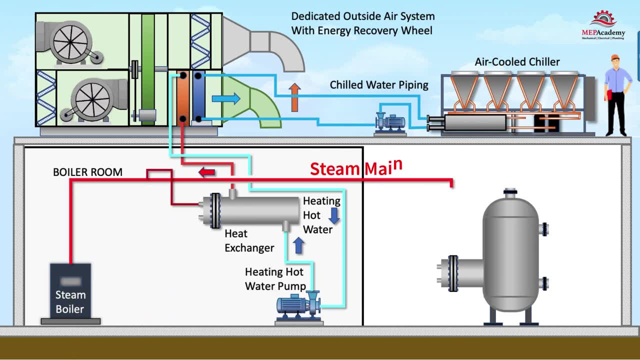 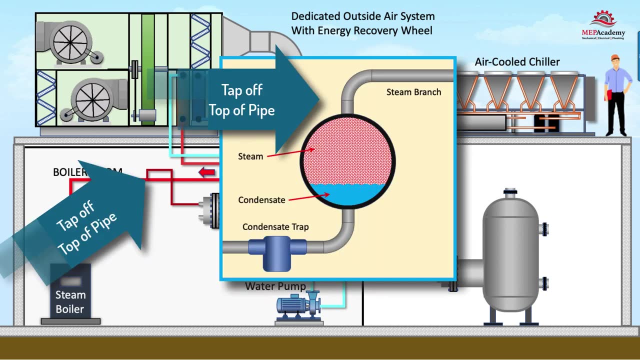 hot water heater and storage tank. We'll have to redo the steam piping to make connections to the domestic system. We'll install a new steam main and make a connection to the heat exchanger, making sure to come up the top of the steam main, which we'll explain why in a minute. 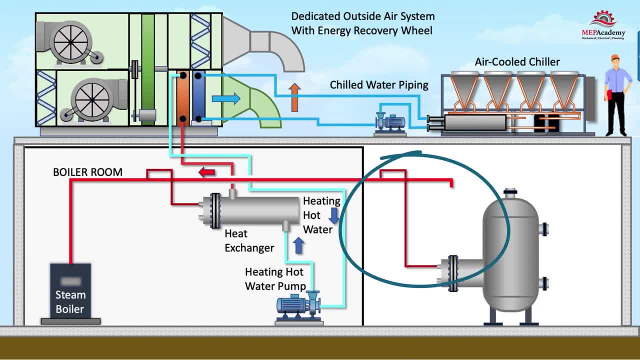 Next we'll connect the domestic hot water heater to the steam main. The domestic hot water heater and storage tank will need a steam trap at the end of any main steam run to allow only condensate to pass through. A main condensate pipe needs to connect all the condensate from any steam system here. 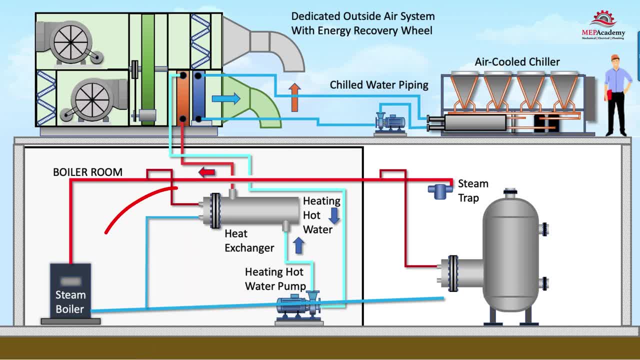 we show a simple system. Next, we'll connect the condensate from the heat exchanger to the main condensate line and be sure to install a steam trap to prevent steam from escaping. allowing steam to escape would be a waste of energy. We will also connect the condensate from the heat exchanger. that 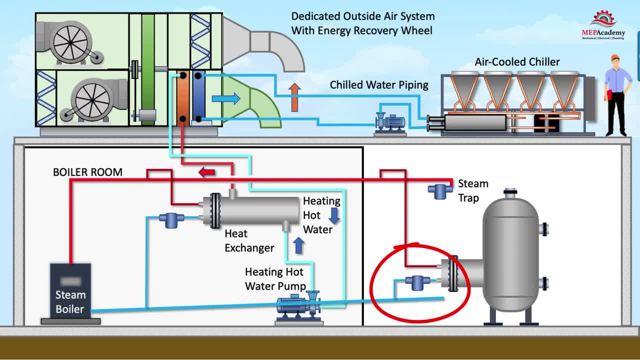 feeds the domestic hot water system and include a steam trap. We need to connect the steam main through the steam trap to the main condensate piping. going back to the boiler, Now we can feed the building with domestic hot water, including a return line, and make up water. 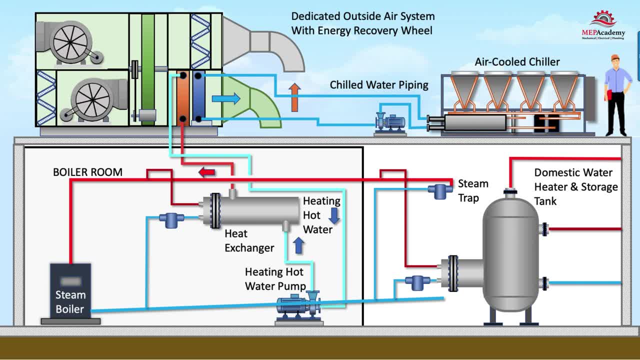 This completes a simple layout of a steam heating system. Of course, there are many other components to a steam system which we will cover in a more advanced video on steam heating, but this gives you a simple view of what it might look like. 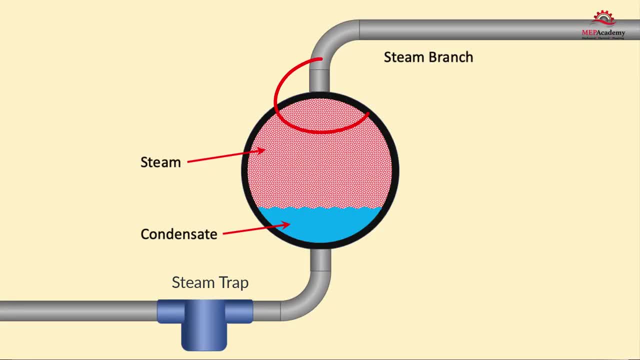 It's important that any steam branch line be taken off the top of the main steam pipe in order to prevent pulling condensate into the branch. As you can see, the steam will rise to the top because of its lighter density and higher temperature. For similar reasons, 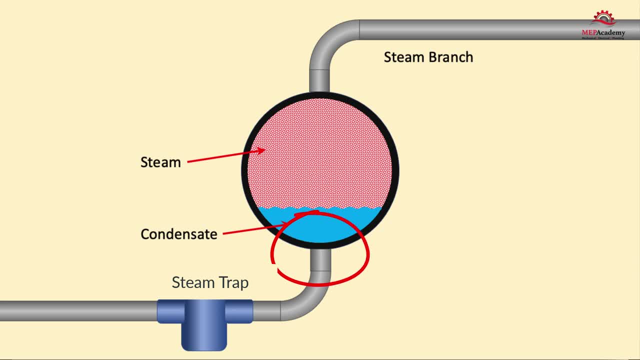 you want to make any condensate that is not in the main steam system. If you have any condensate, branch connections off the bottom of any steam line or system to ensure that you are only pulling condensate, and all condensate branches should contain.